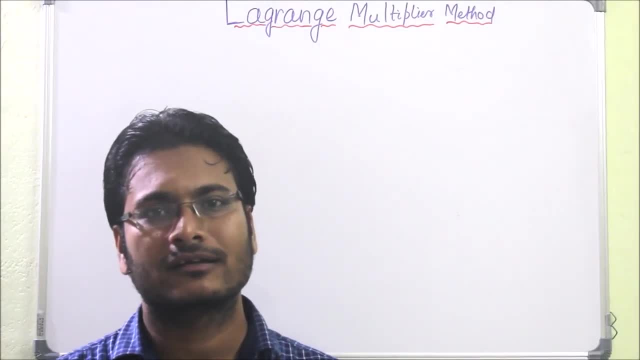 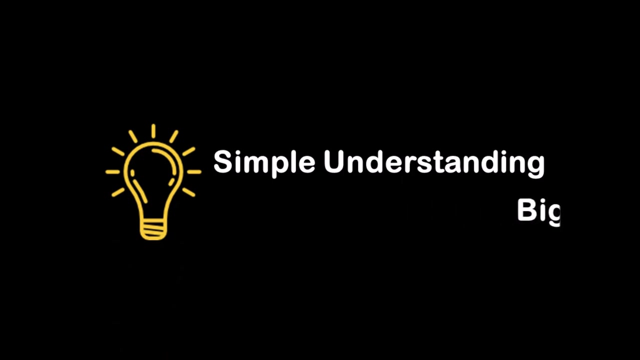 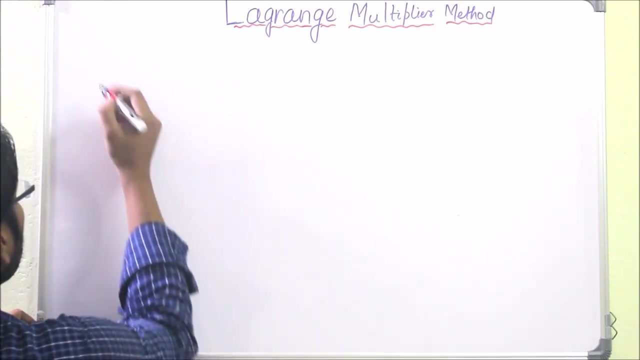 Today we will see one of the most popular method, that is, Lagrange multiplier method, to find the minimum or maximum amount of multivariable optimization problem with equality constants. So let us start with the statement, then we will see how to find the minimum or maximum of problem. 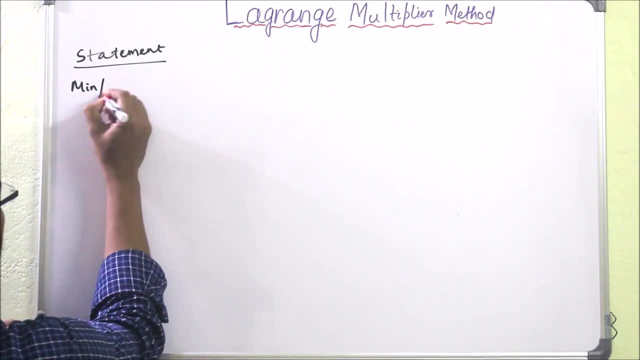 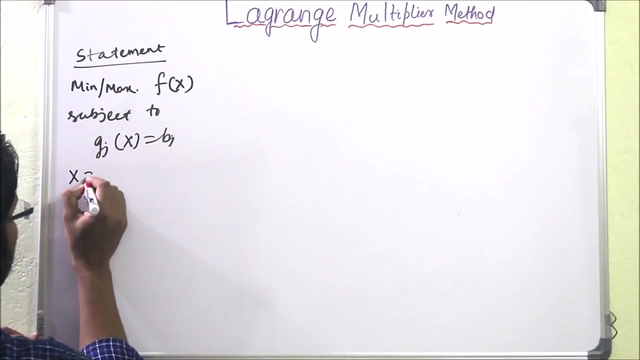 So the statement is that we have to find or minimize or maximize f of x subject to gj, x equal to bj. So we will see what is x and what is j. x is nothing but n component factor, x1, x2 up to xn. 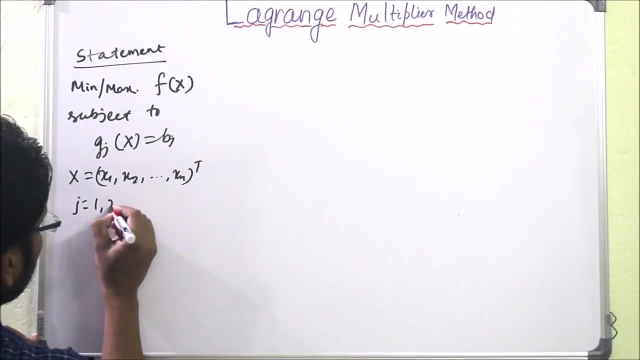 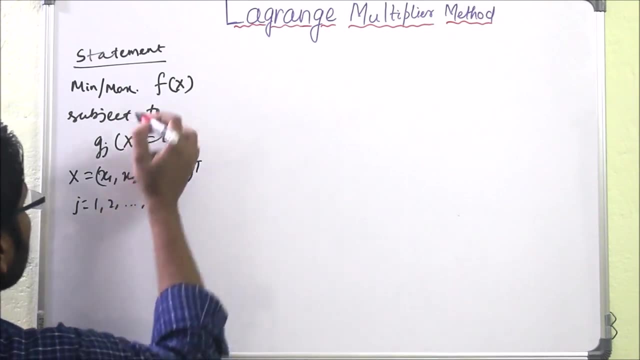 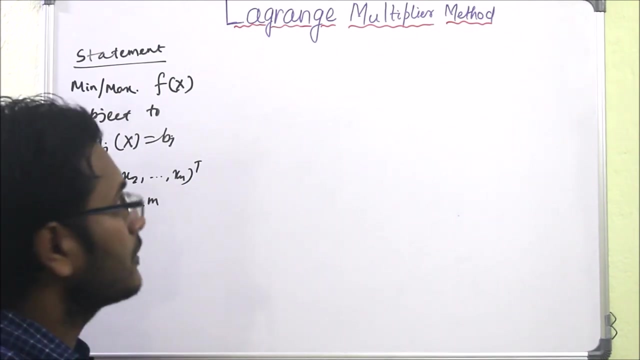 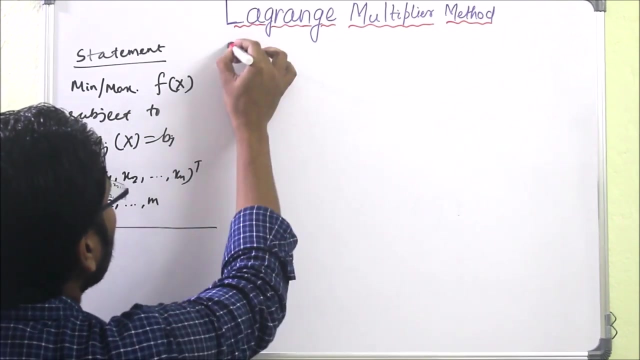 And j is running from 1 to m And there are m equations, m equality constants. So this is the statement of the problem. Now, how to find the minimum or maximum using Lagrange multiplier? that we will see. So, as I have told, the strategy for all the equality constant problem is same, that is, we have to convert. 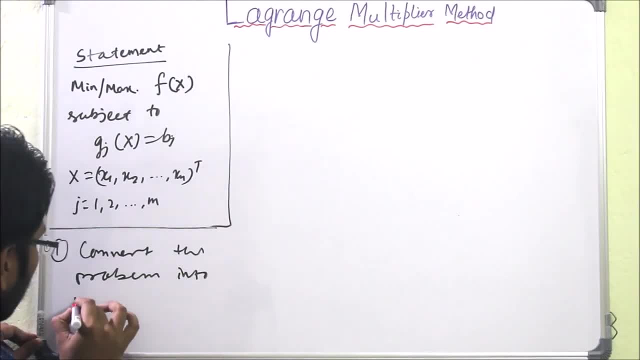 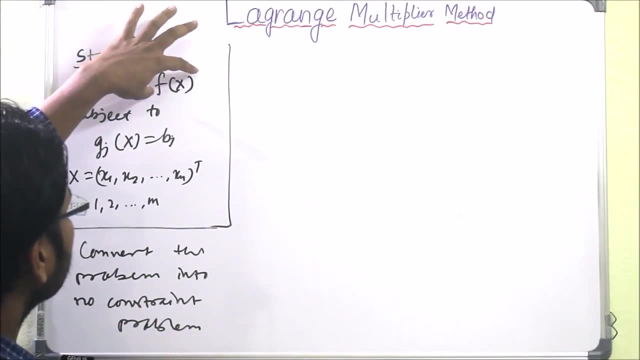 the problem into no constraint problem, Then what will happen? then the original objective function will change into new objective function And that will give the problem. that will give the multivariable optimization problem without constant. So how to do that, we will see. So, as we have m equations, 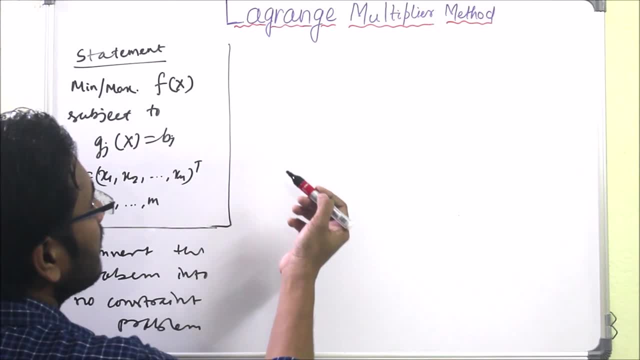 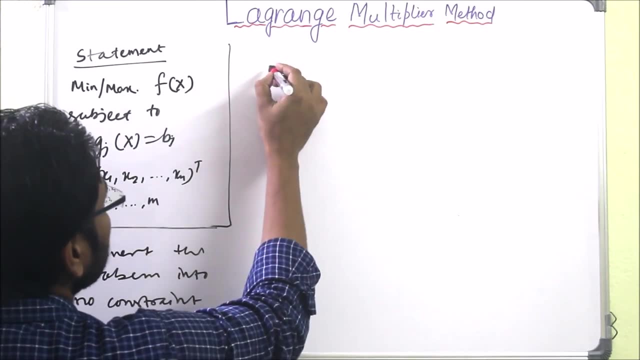 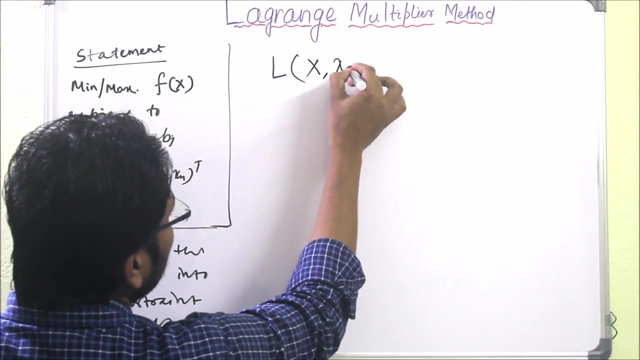 So for m equation we will take m multiplier, that is lambda 1, lambda 2 up to lambda m. So this problem will change into this form. That means our new objective function will be: L of x, lambda 1, lambda 2 up to lambda m. 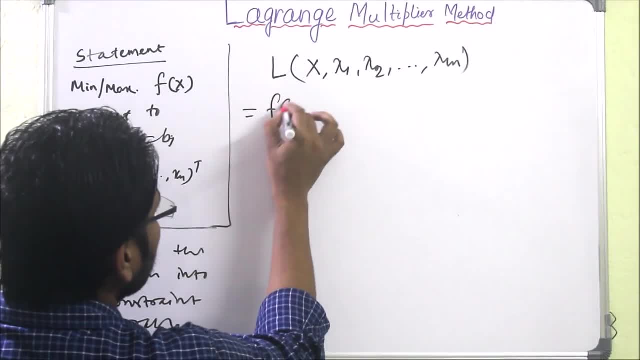 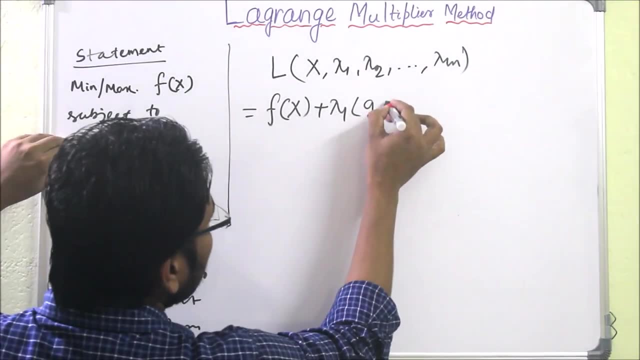 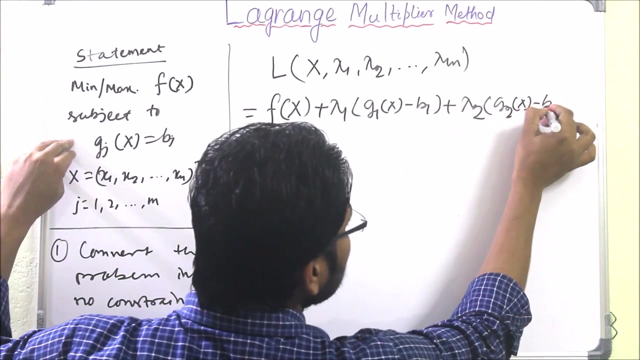 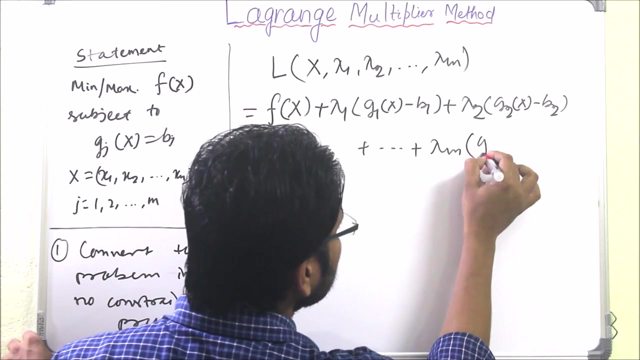 So how to write this? This will be nothing but the sum of this f of x plus lambda 1 times lambda 2.. This g1 x minus b1 plus lambda 2 times g2, x minus b2 plus, and so on, And last term will be lambda m, gm x minus bm. 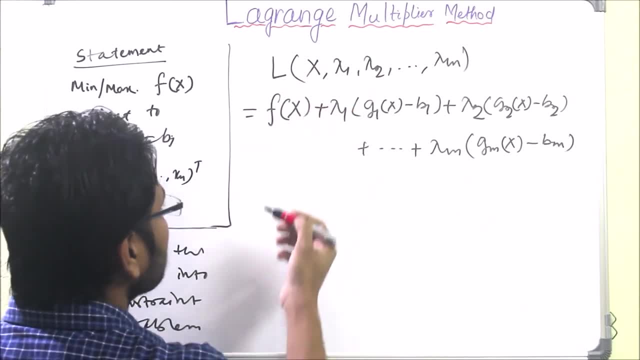 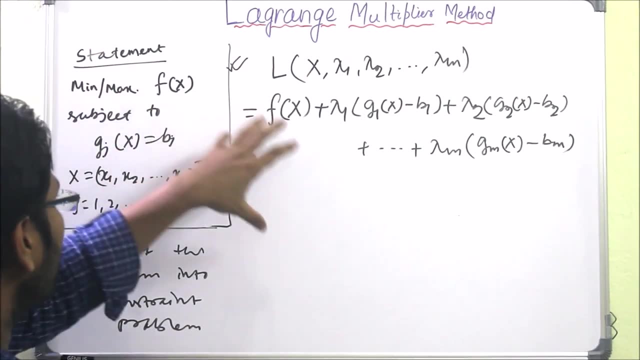 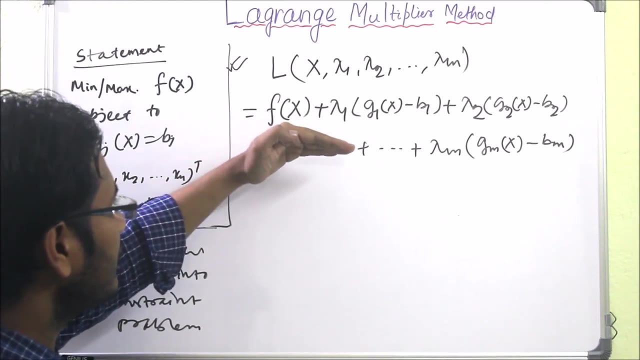 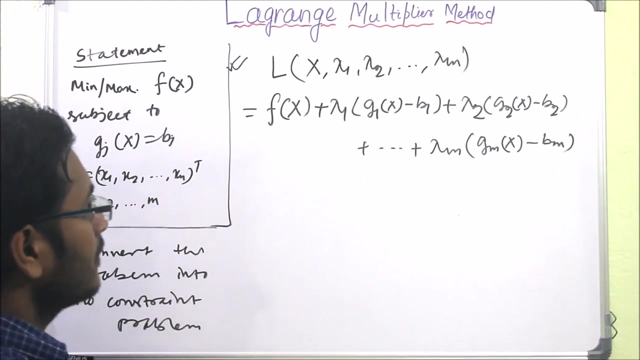 So here x is nothing but n components. So this is the modified version of the objective function. By this way we can convert this equality constraint problem to without constraint problem. So after that, what is the approach? The approach is same, like the approach we have followed in multivariable optimization without constraint. 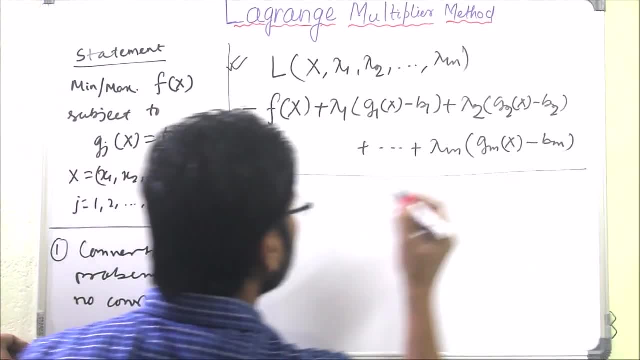 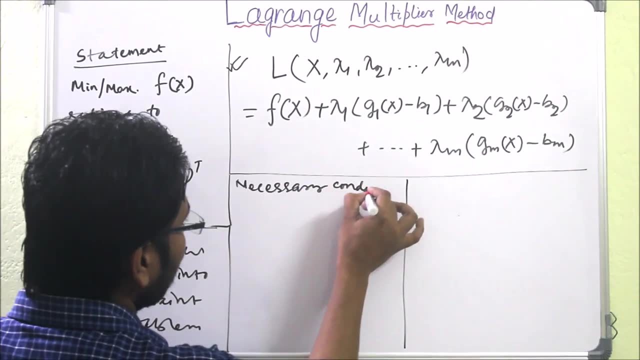 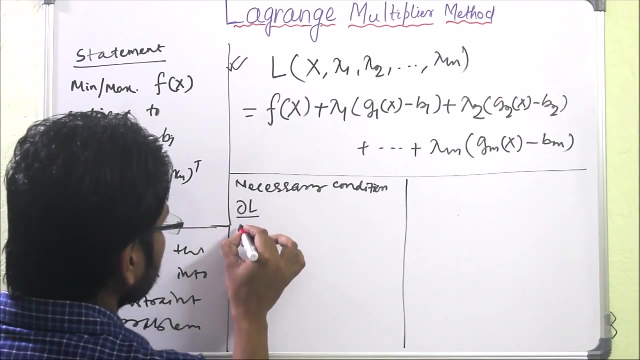 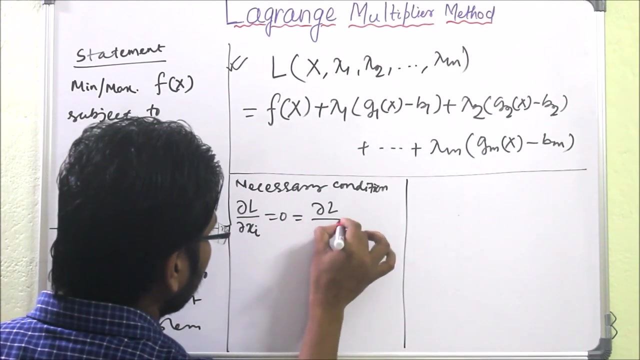 So what to do? We have to do in two ways. that is, first we have to see the necessary condition. So what is necessary condition, Necessary condition, says that its first order partial derivative will be 0. That means del L by del x, i will be 0 and del L by del lambda j, I can write. 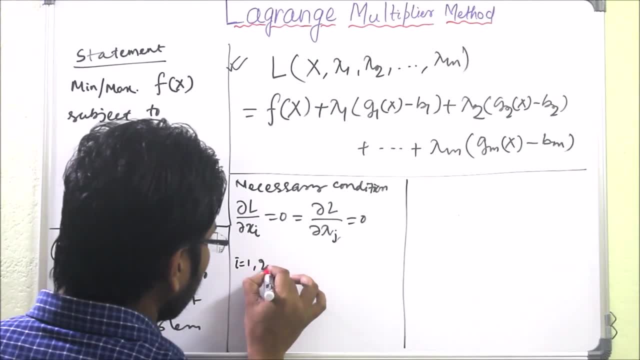 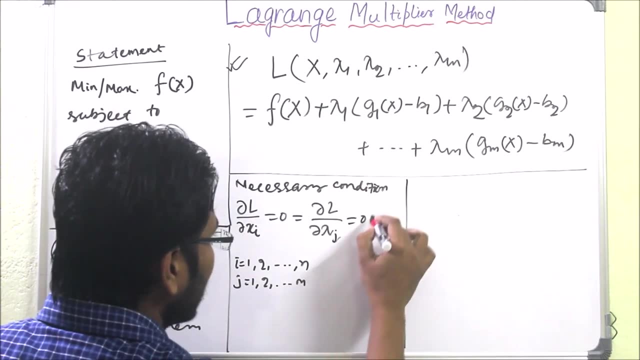 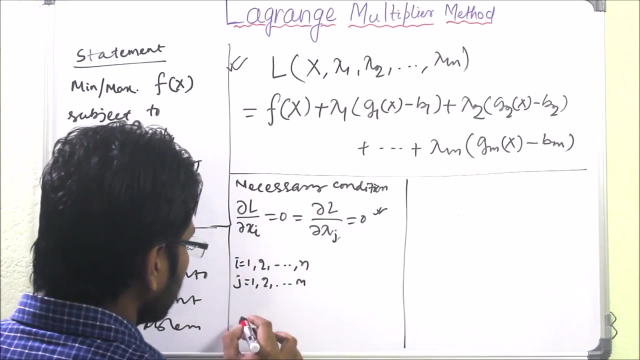 lambda j equal to 0, where i varies from 1 to n and j varies from 1 to m, So that we have to see. So after that, what we have to do: After equating all those first partial derivatives, we will get this: x i value and lambda j value. 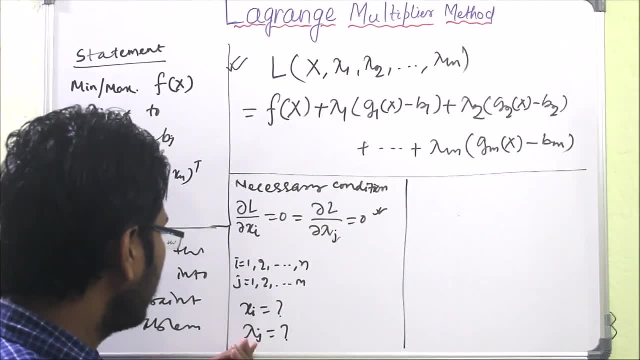 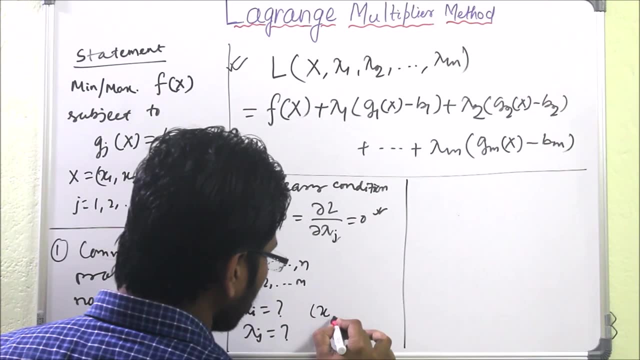 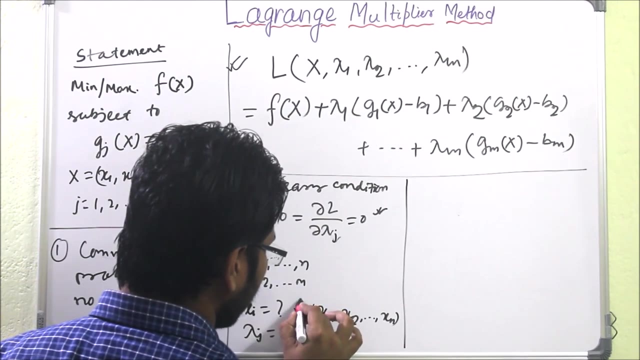 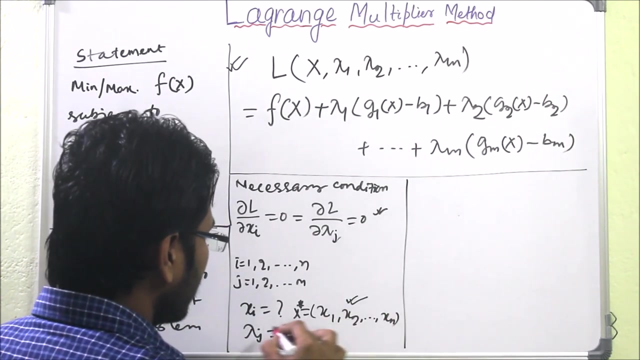 So after getting all this value, x i lambda, j- we can say that what is the x1, x2, xn? Okay, So what is x star? X star means the extreme point. So by equating all those things, whatever combination we get for x i value, that will give the extreme value. 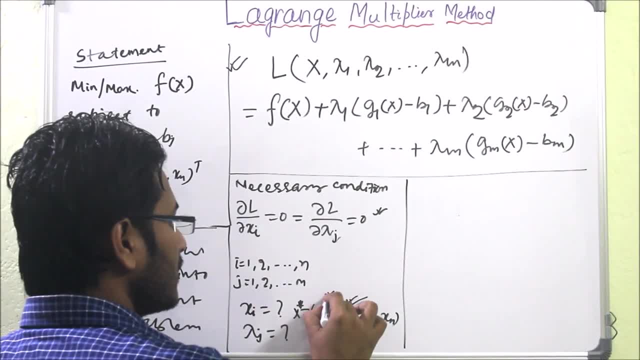 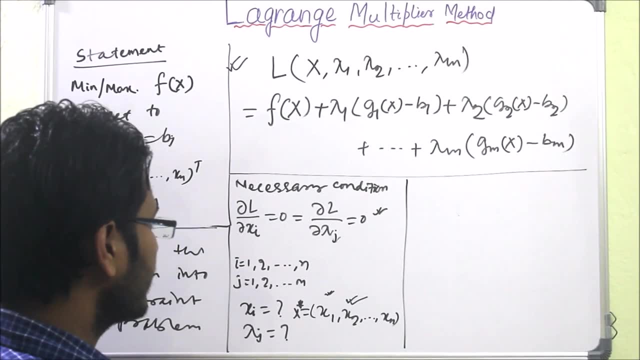 Okay, That means that point. at that point the function value will be extreme Means: either maximum means relative maximum or relative minimum. Okay, But how to know that at this point it will be Relative minimum or relative maximum that we can see through the sufficient condition? 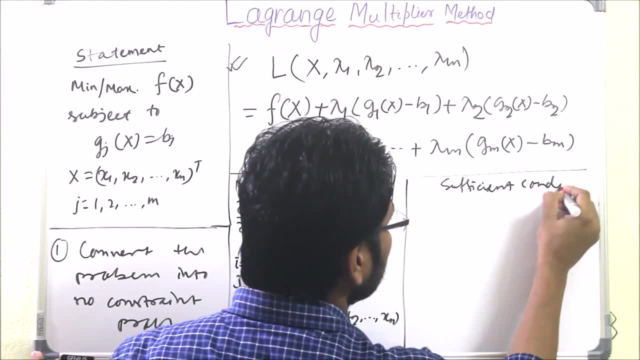 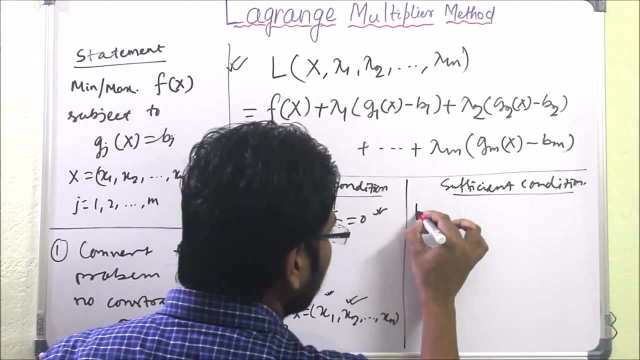 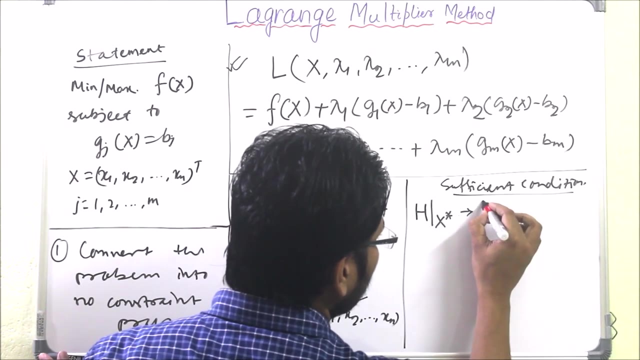 Okay. So how to find sufficient condition? We have to find: if x star is a point. Okay, Then we have to find the Hessian matrix at x star. Then we have to see: either it is positive, definite. If it is positive, definite. 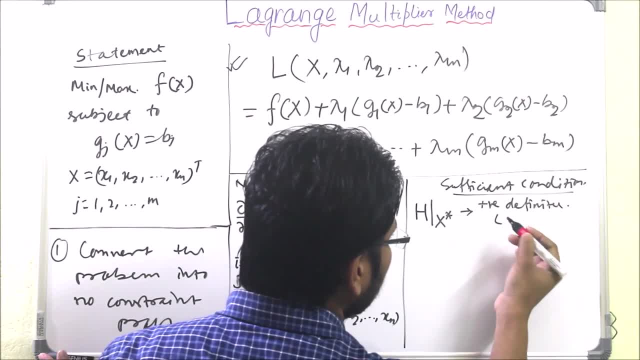 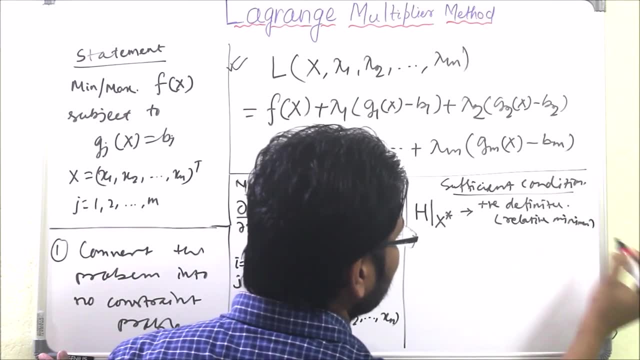 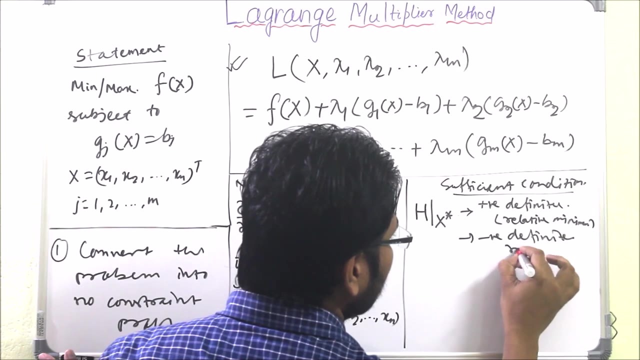 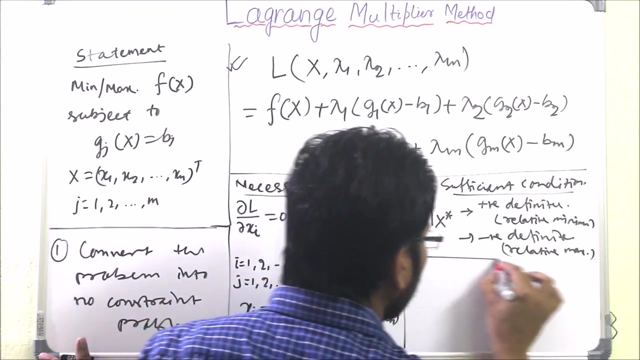 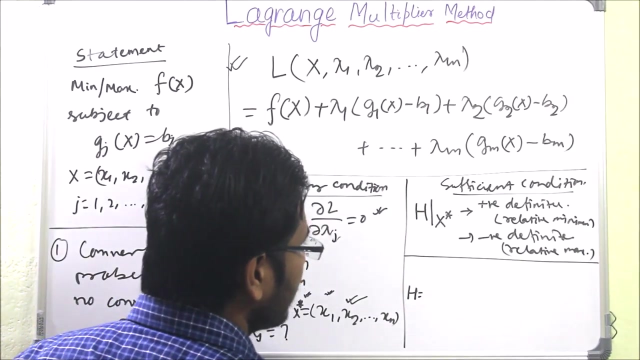 Then what x star, having the? what relative minimum at that point? Okay, If it is negative, definite, then relative maximum, Otherwise it is a saddle point. So how to write the Hessian matrix? So Hessian matrix is nothing but The second order, partial derivative of all those, the independent variables. 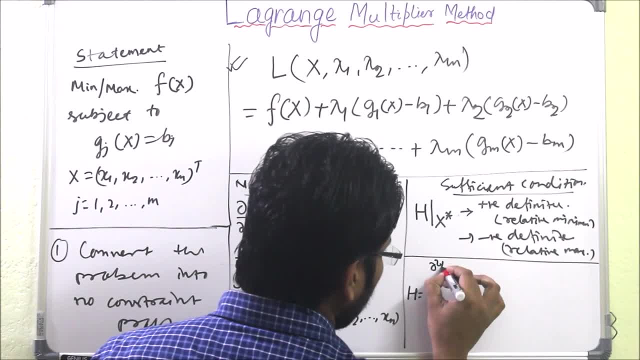 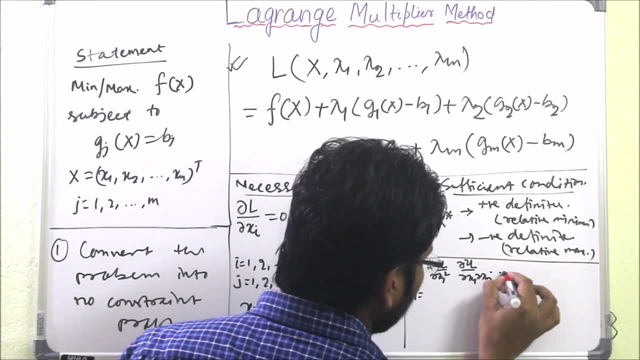 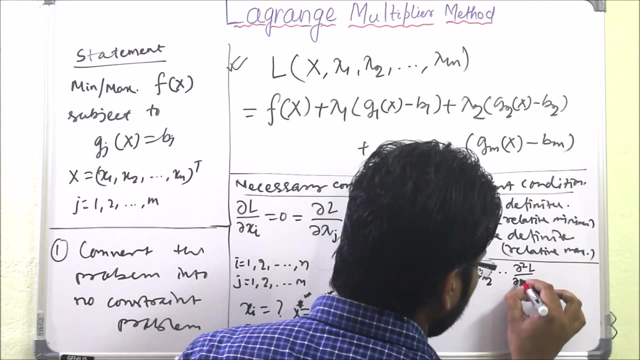 So h will be del two l by del x one square. Del two l by del x one del x two, Like that it will go. Then after some time it will be means after n time it will be del two l by del x one del lambda one. 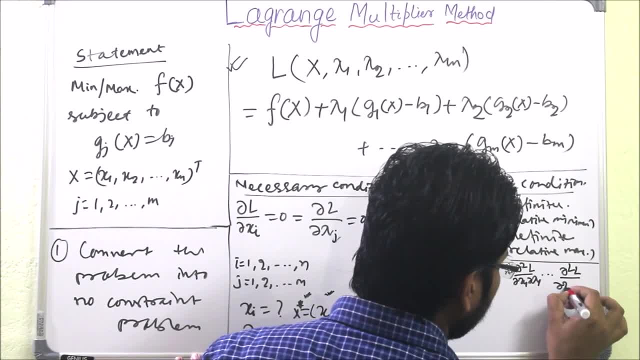 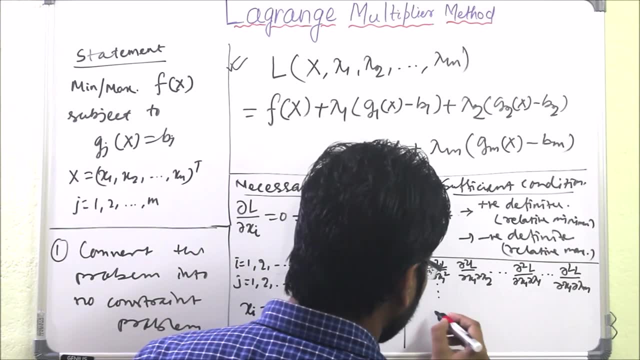 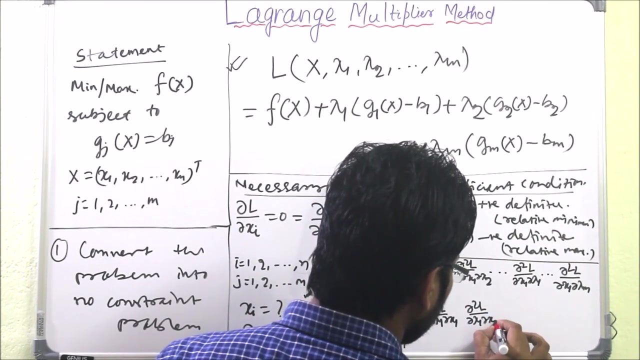 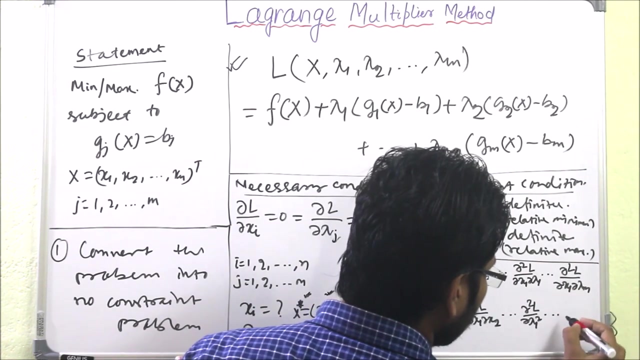 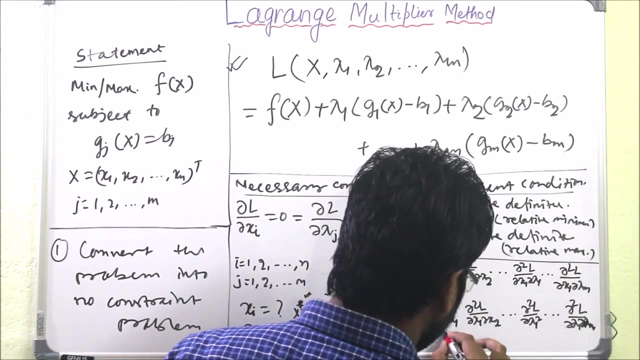 Simply then it will go. Then, finally, del two L by del lambda one square, And then del two L, three by Stacy. Now delta two, cool, And then delta two L by delta one, Okay, And then del lambda 1 square, and then so on, del 2 L by del lambda 1, del lambda m and last term. 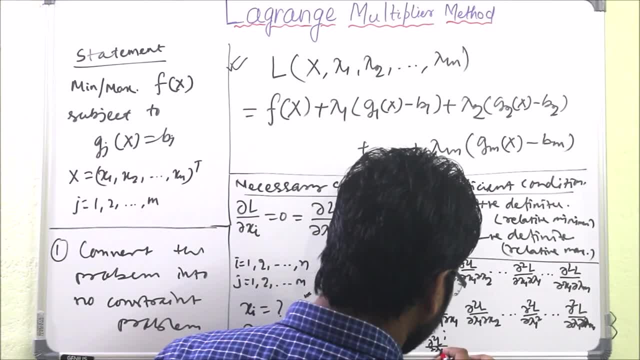 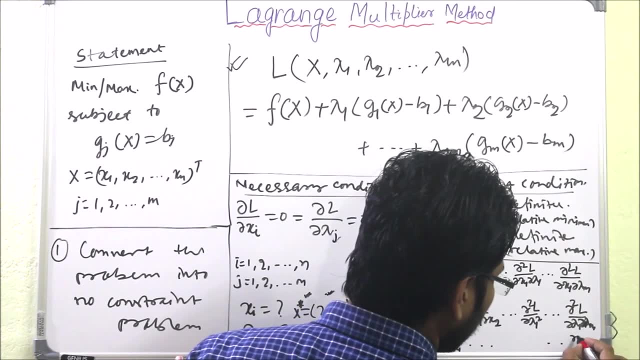 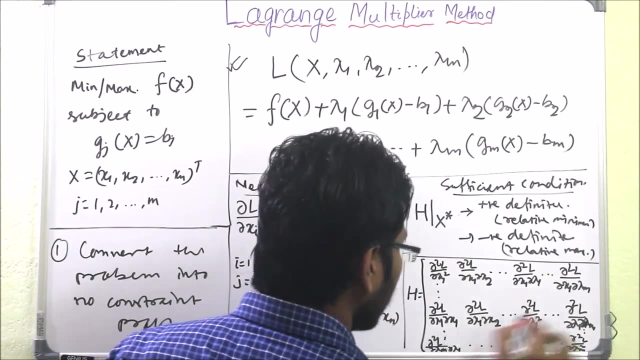 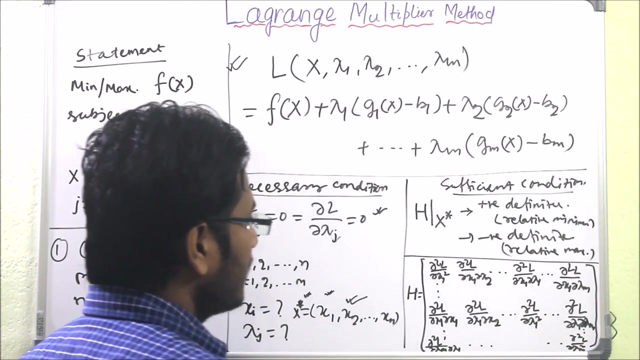 will be del 2 L by del lambda m, del lambda 1 and so on. so on, last element will be del 2 L by del lambda m square. so this is our axion matrix. then we have what we have to do. we have to put the x star value here and we have to find whether the x matrix is positive.